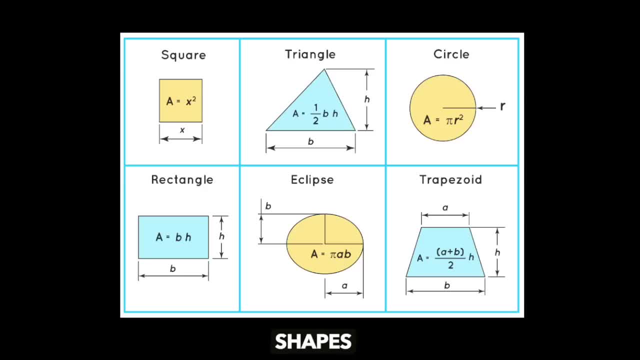 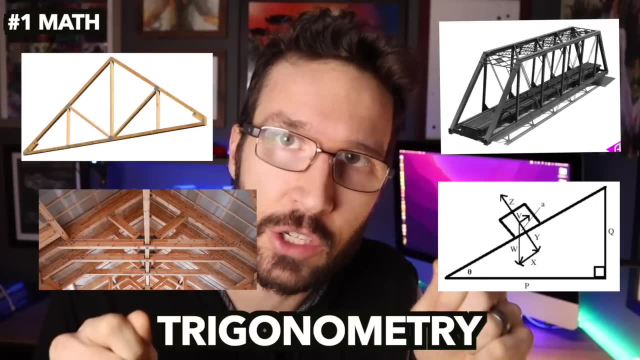 Next up, we have trigonometry. In trigonometry, you're going to learn all about shapes and ratios and angles, right, But most importantly, you're going to learn about triangles. Triangles are everywhere in engineering, especially in mechanical engineering. 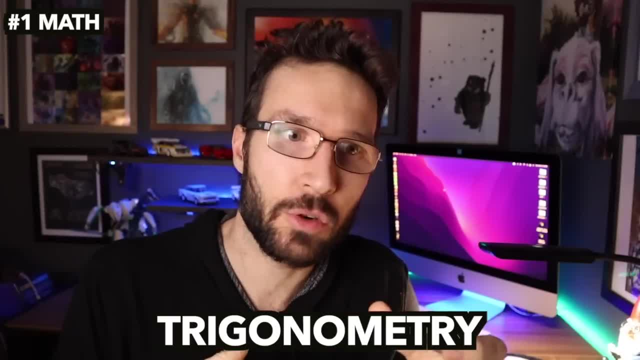 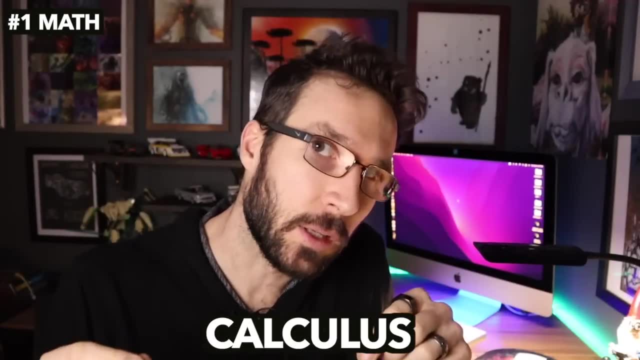 So in trigonometry you'll really learn all the tools and different tricks and equations that come with triangles to solve all sorts of engineering problems. Next up we have calculus, Calculus, Calculus, Calculus, And in mechanical engineering you're going to have to go through calculus one, two and three. Just a heads up. 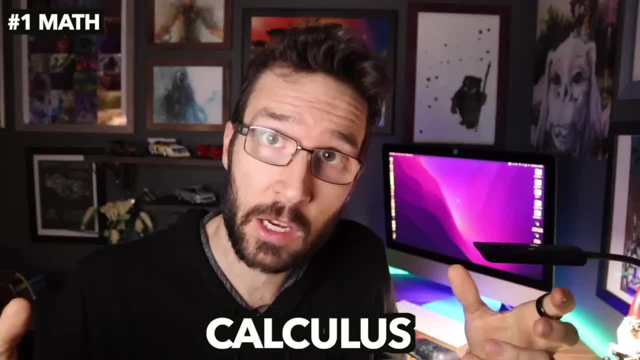 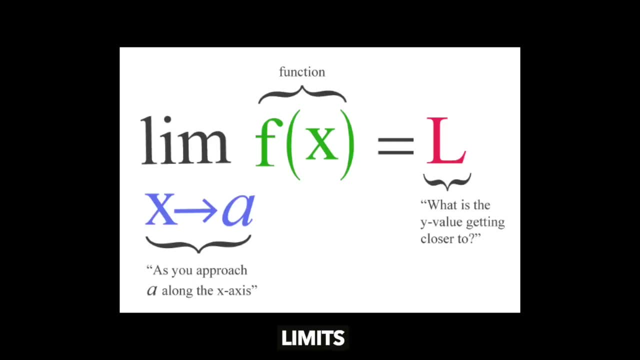 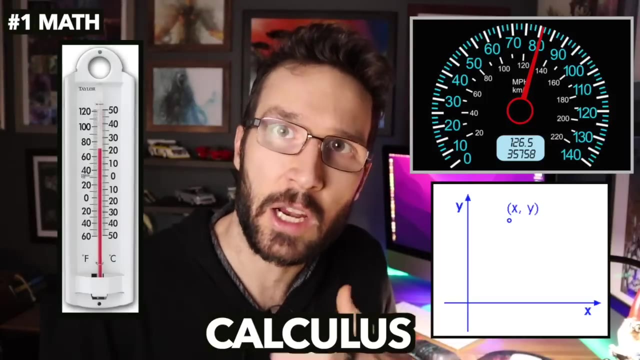 So calculus is the branch of math that deals with continuous change, right, Continuous position change, temperature change or time change. You're going to learn about integrals, derivatives and limits. These tools are going to allow you to solve problems where variables like speed, position and temperature change with time. 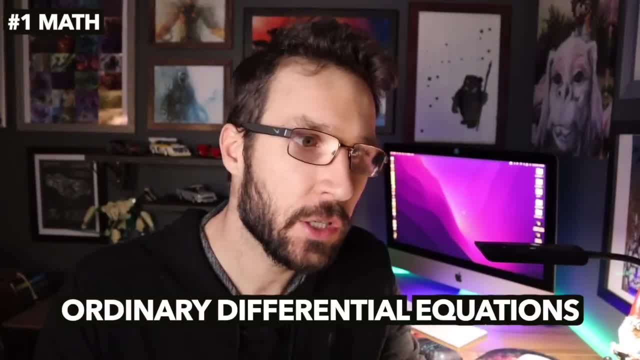 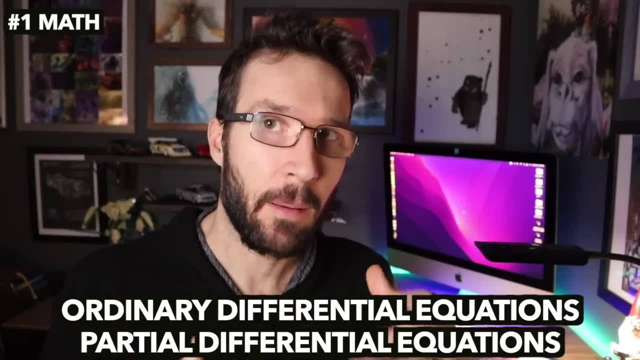 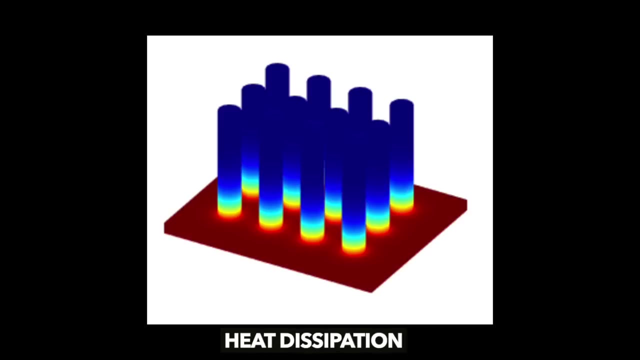 And lastly, in math, you're going to learn ordinary differential equations and partial differential equations. So these These high-level math courses are going to teach you how to model and predict how moving physical systems will behave into the future- Things like oscillation, wave behavior and heat dissipation. 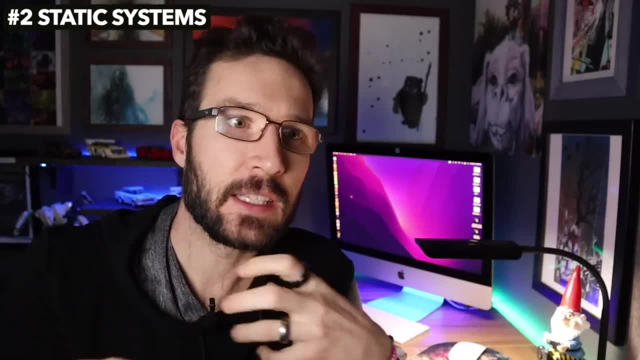 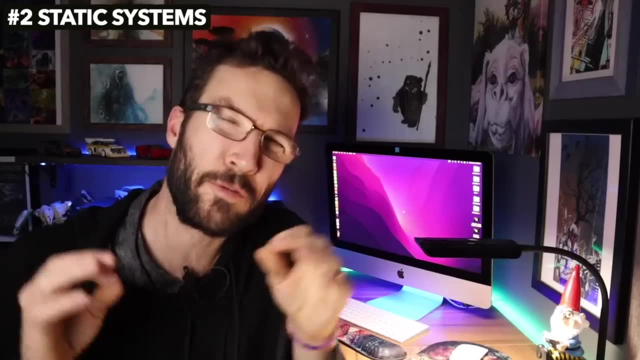 Category two: static systems. So just to clarify, a static system is just something that's unmoving, right? It's not moving, It's like a bridge or a column or a beam. So the first course in this category is physics, Physics one. 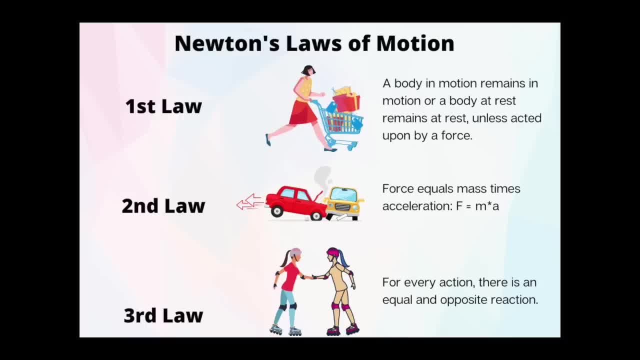 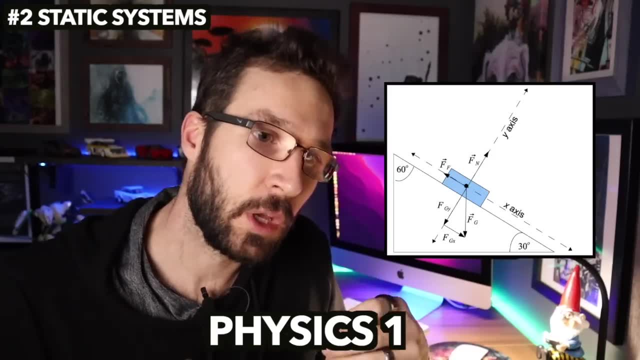 So in physics one, you'll learn all about Newton's laws of motion and how to apply it. You'll learn about momentum, gravity, friction and velocity, And you'll learn about how to utilize trigonometry to determine the forces and angles of those forces on a given object. 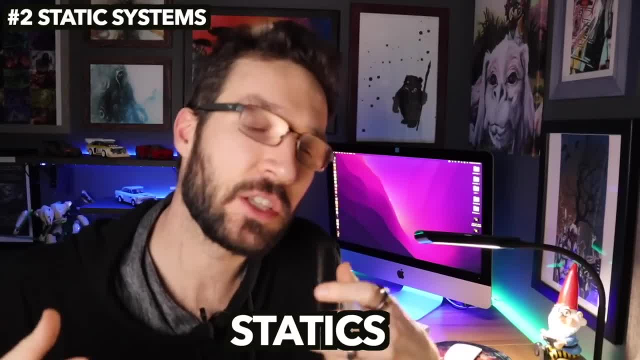 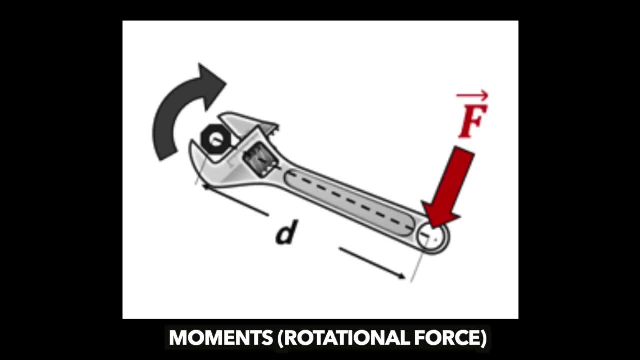 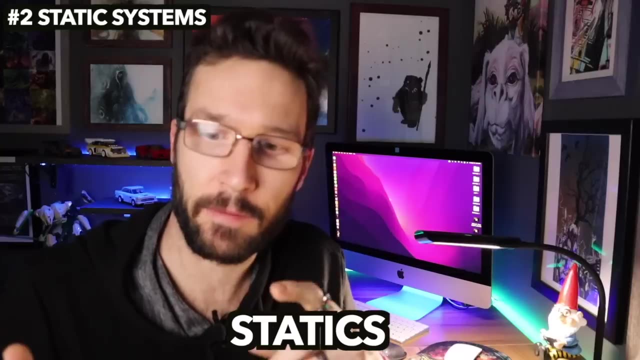 The next course is statics. So in statics you're going to dive much deeper into the analysis of static systems. Some of the topics include force vectors, moments or rotational force, center of gravity, friction, force balancing and just a much more in-depth analysis of. 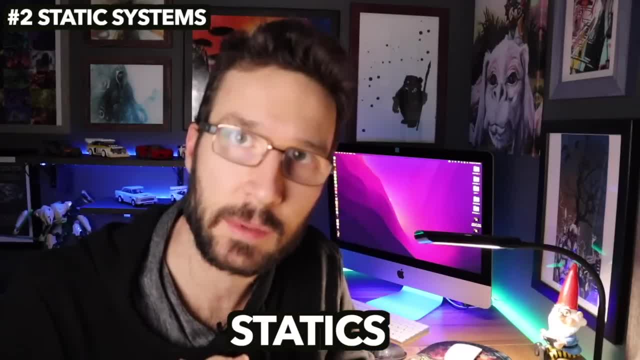 and just a much more in-depth analysis of, and just a much more in-depth analysis of, beams, trusses, columns and a lot of other static systems. Hey, I hope you enjoyed the video so far. If you are, make sure you hit the like button, subscribe to the channel and share it with your friends. 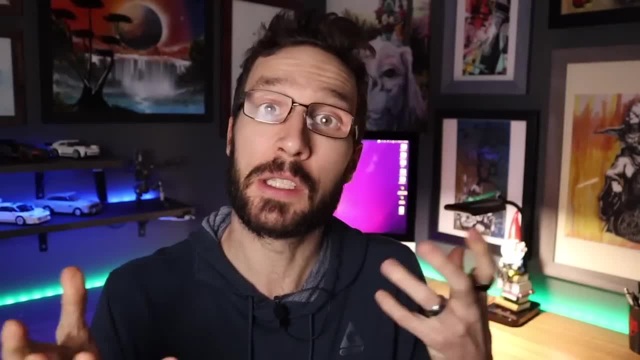 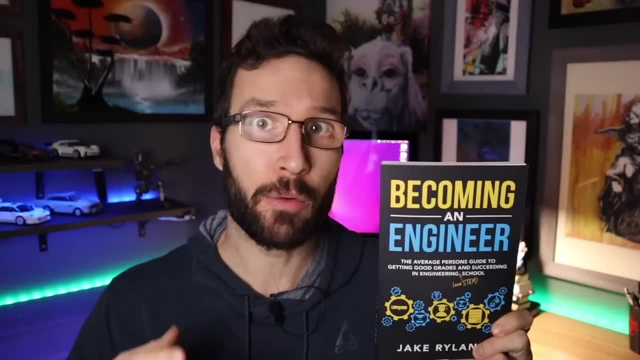 That kind of stuff really helps the channel grow, And if you or anybody you know is looking to study engineering or any other STEM degree, be sure to check out my book. You know I wrote this book to serve as a true universal guide, right? 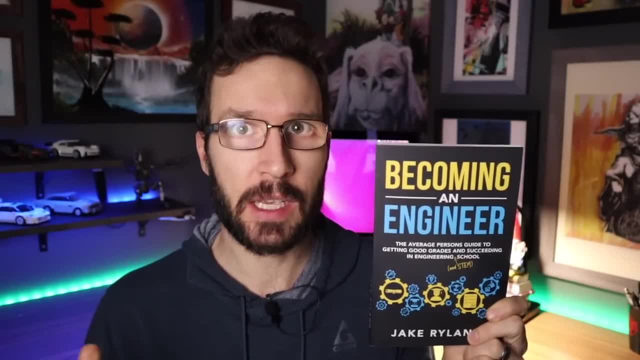 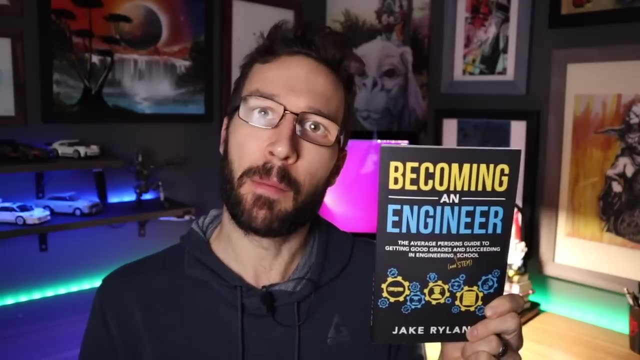 A roadmap to show how anybody and everybody can have success in engineering or any other STEM degree. It's getting great reviews so far. You can go on Amazon and see for yourself. It's available in paperback, ebook and audiobook, So I'll put links in the description for everything. 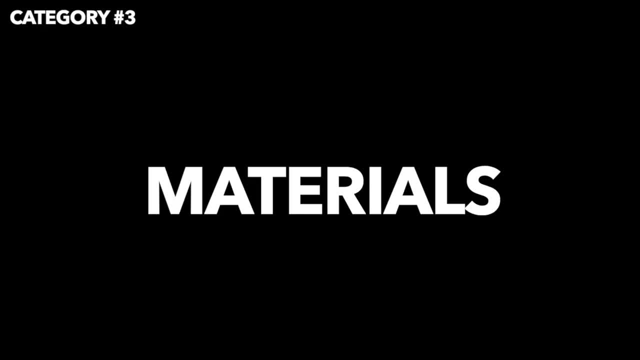 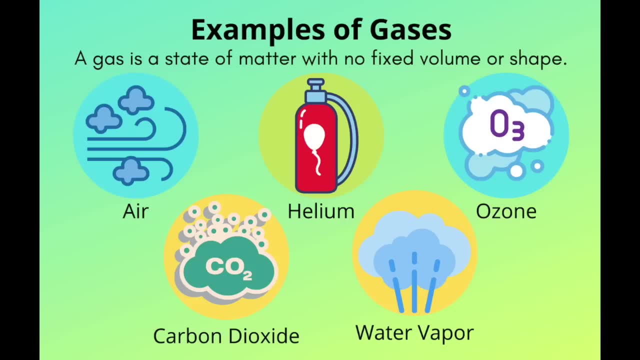 Thanks for the support Category number three: materials. So first up in this category we have chemistry. So in chemistry you're gonna learn all about the periodic table of elements: Liquids gases, solids, right Storchiometry. 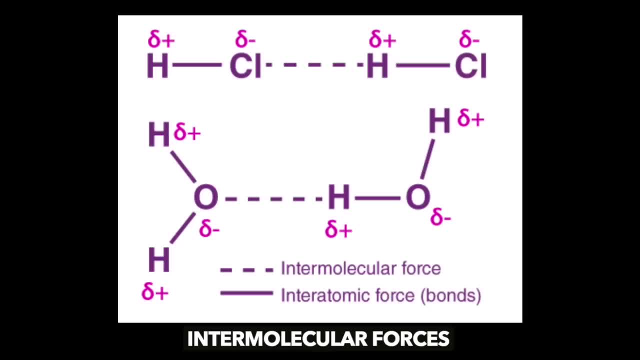 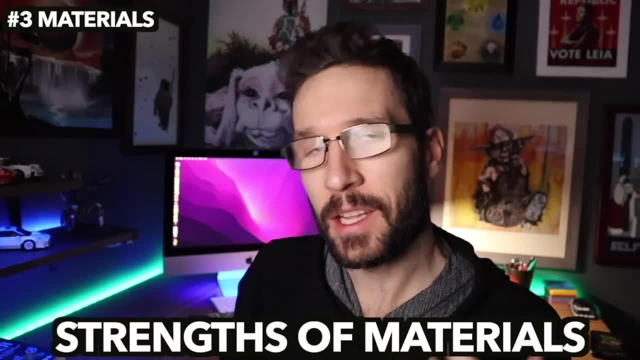 You're gonna learn about bonding and intermolecular forces and structure, And then you also learn how to balance chemical equations. Next up we have strengths of materials. So in strengths you're gonna learn all about how different materials and shapes deal with stress and strain, right? 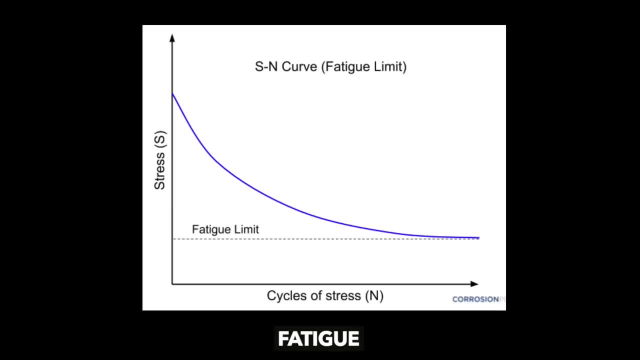 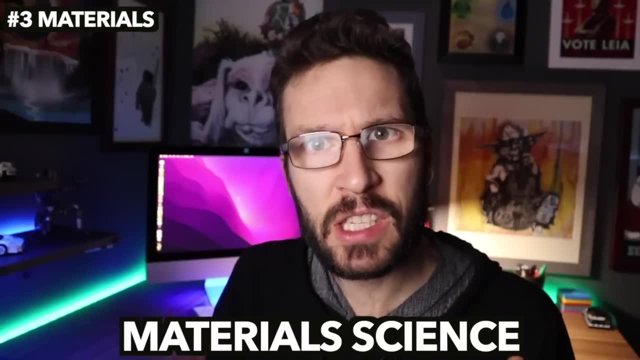 So other topics include plasticity, elasticity, fatigue creep yield and material failure. So last up in this category we have material science. In material science you're gonna dive much deeper into the structure of materials. You're gonna learn how to predict the properties. 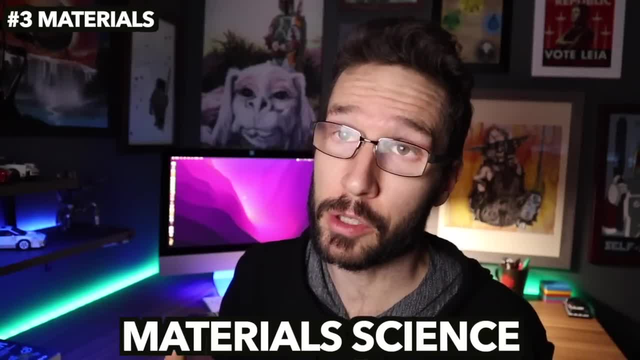 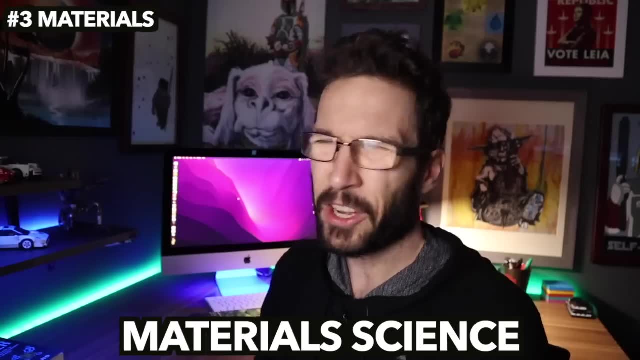 and behavior of a given material based on its microstructure. You'll also learn about atomic bonding, melting point, thermal expansion, crystalline materials and diffusion, And you'll also learn about what controls the electrical, optical and thermal behavior of a given material. 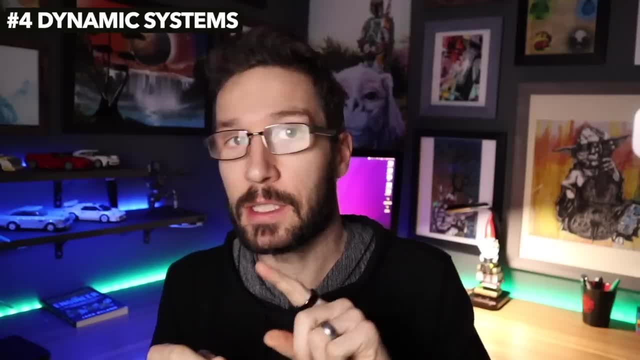 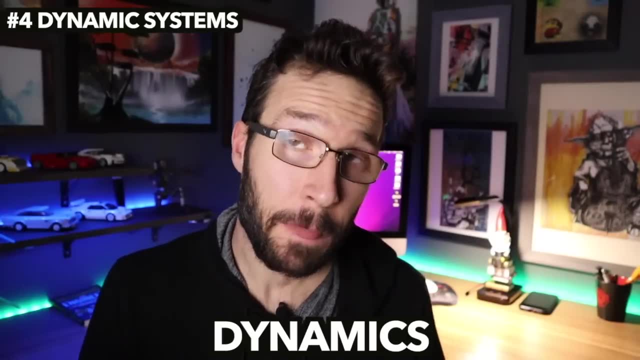 Category four: dynamic systems. So static systems are things that aren't moving. Dynamic systems are things that are moving. So first up in this category we have dynamics. In dynamics, you're gonna really expand pretty thoroughly on what you already learned in physics one. 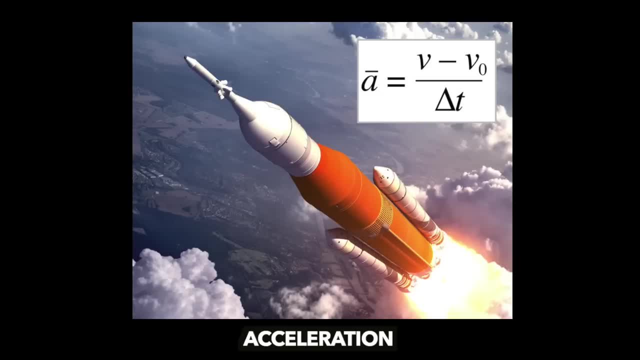 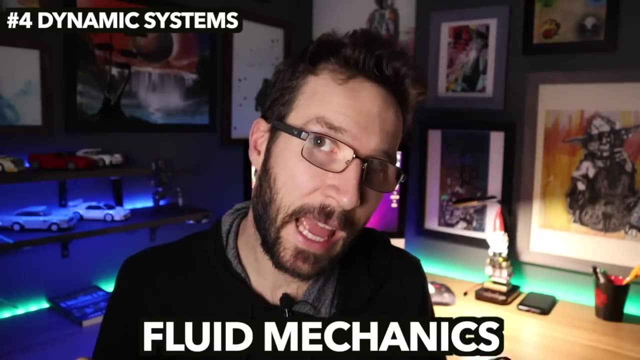 So topics include kinematics, velocity, acceleration, momentum, vibrations, impacts and energy. Next up, we have fluid mechanics. This is one of my personal favorite courses, by the way, So in fluid mechanics you're gonna learn all about. 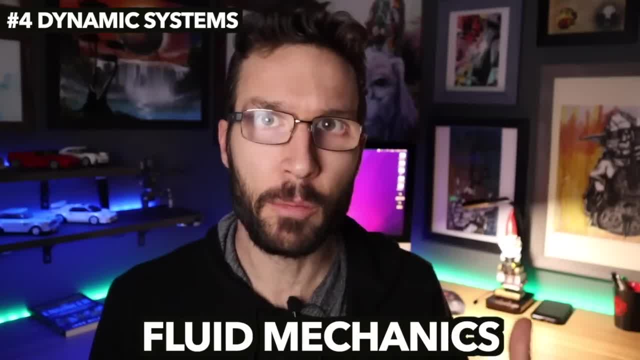 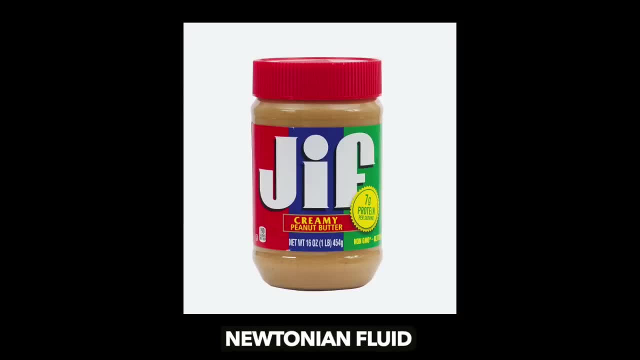 how different fluids move and behave in different environments. right, So you're gonna learn all about fluid kinematics, hydrostatics, Newtonian and non-Newtonian fluids, boundary layers, laminar versus turbulent flow, and conservation of mass and momentum. 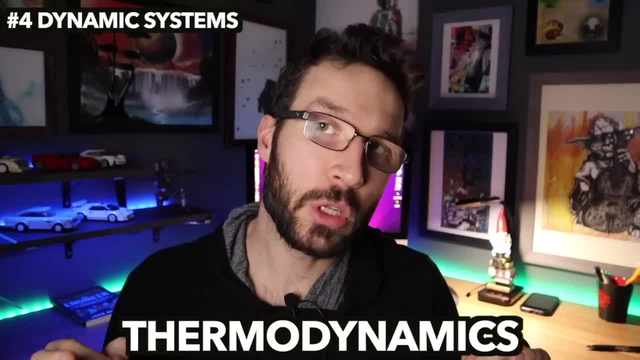 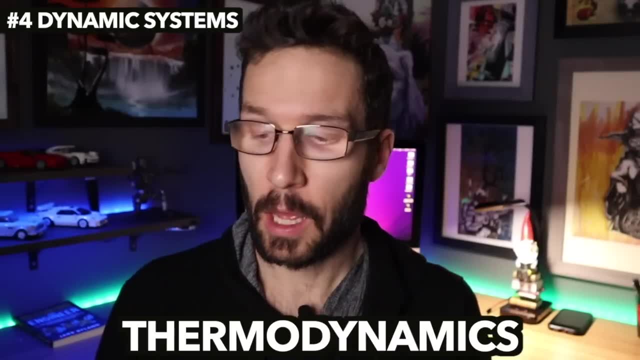 So next up we have thermodynamics. In thermodynamics, you're gonna learn all about energy and how it's used, and how it's used in the environment, How it's used and utilized to make things work right. So the topics include energy cycles, engines, heat work. 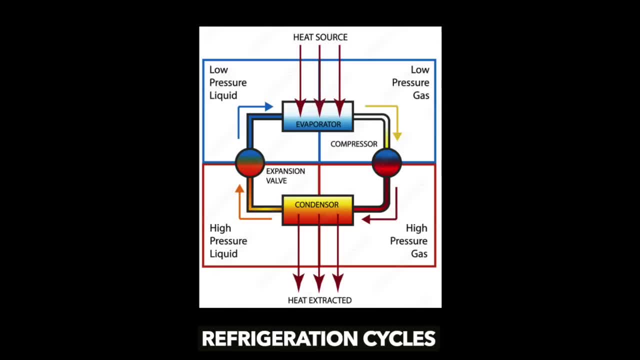 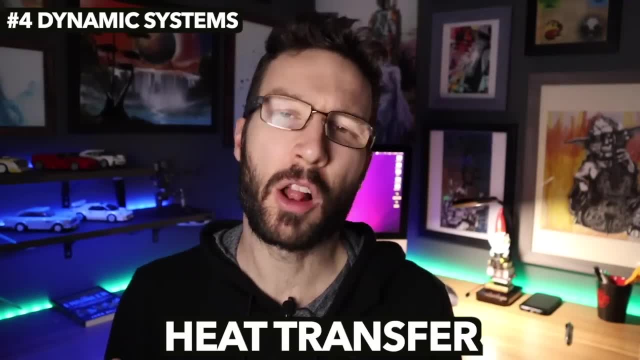 entropy, enthalpy efficiency, refrigeration cycles and conservation of energy. Okay, so last up in this category we have heat transfer. So in heat transfer you're gonna learn all about how heat moves between different mediums, right? 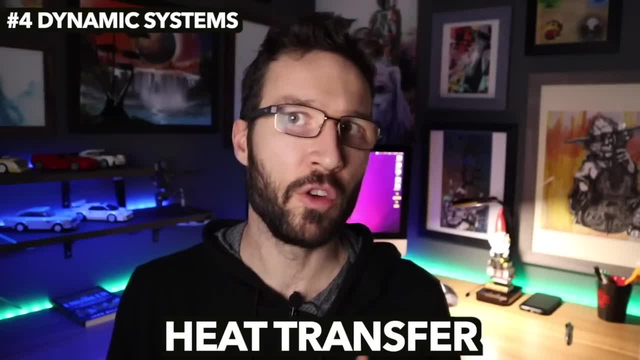 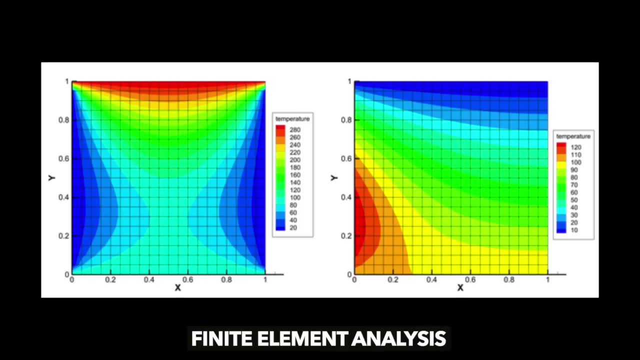 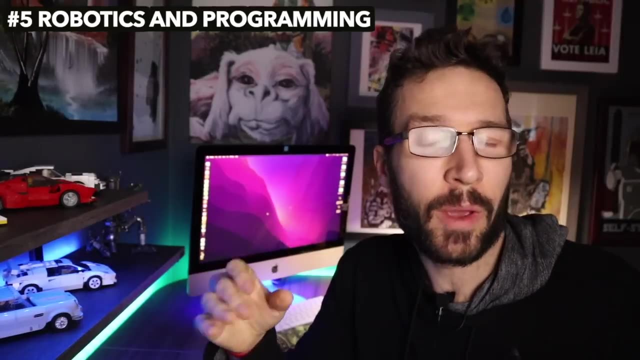 So you'll be able to calculate and predict and eventually control the movement of heat in your design. So topics include conduction, convection, radiation, heat exchange and finite element analysis. Category number five: robotics and programming. So first up in this category we have physics. two. 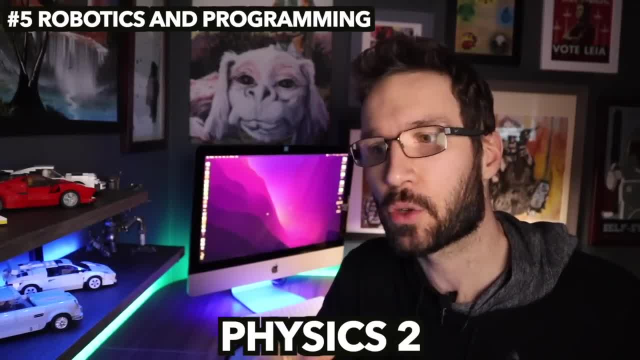 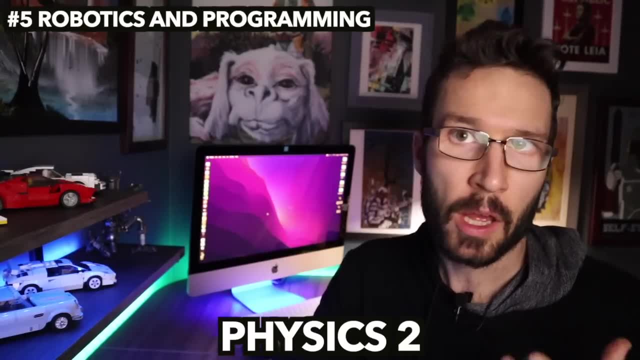 So in physics two you're gonna get a real kind of in-depth crash course into electricity and magnetism and how you can use math or calculus specifically to analyze those things right. So the topics include electrostatics, electric fields and potentials. 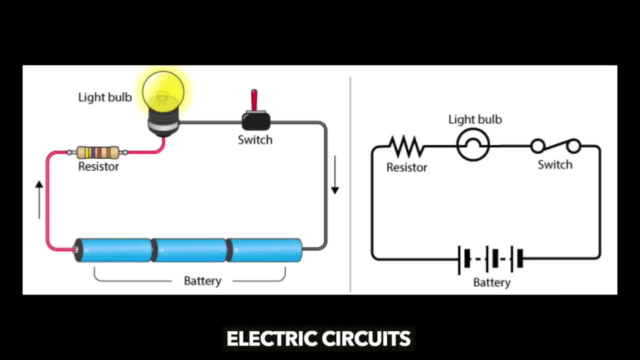 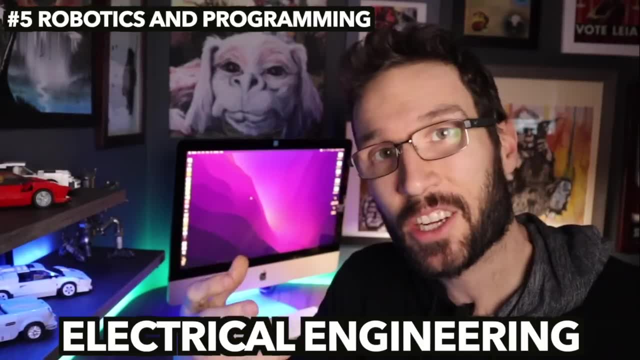 magnetic fields, current flow, electric circuits, resistance, capacitance, inductance, electromagnetism and optics. So next up in this category we have electrical engineering. In electrical engineering you're gonna really build upon the knowledge that you've got from physics. two: 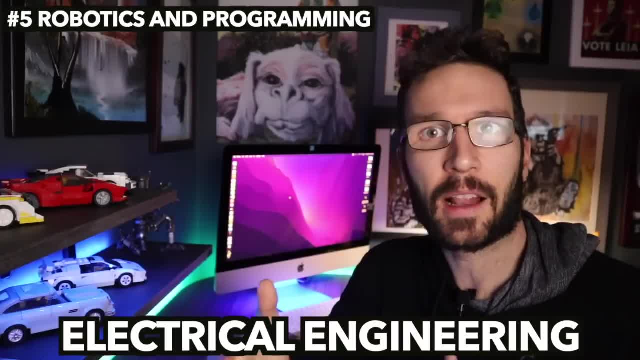 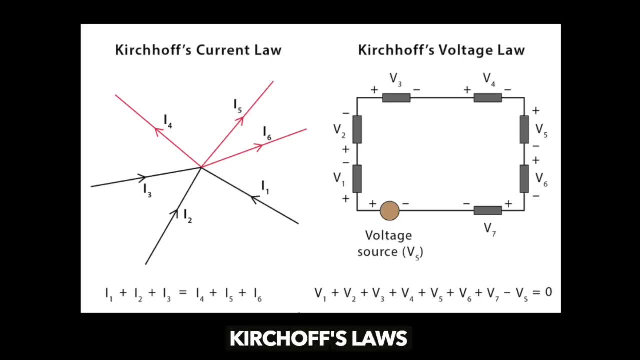 So you're gonna get really more in-depth with electric circuits and how to analyze and predict resistance, current flow, voltage, capacitance, inductance, right. Other topics that you're gonna cover are Kirchhoff's laws, diodes, amplifiers, power actuators and transformers. 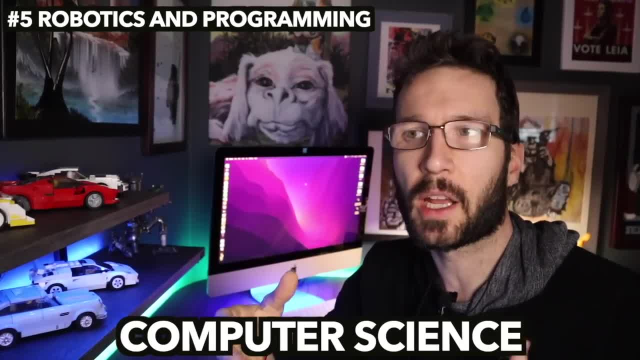 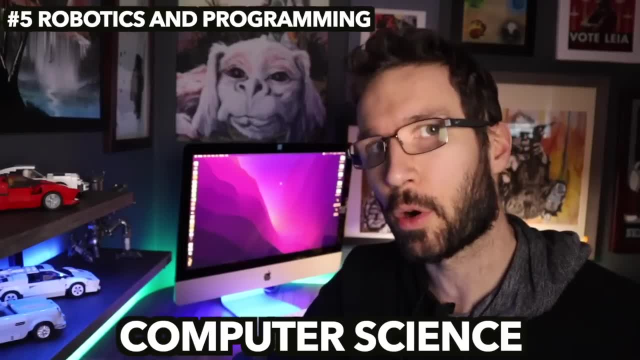 Next up we have computer science. So in computer science you're gonna get a good intro, a good crash course into computer programming. right, You're gonna learn basic coding language and how computers are programmed and execute different commands. You're gonna learn how to create your own programs. 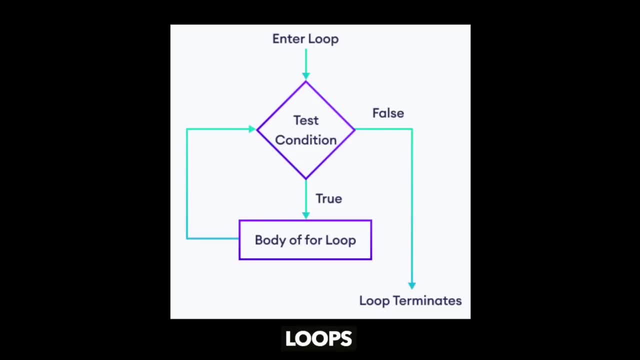 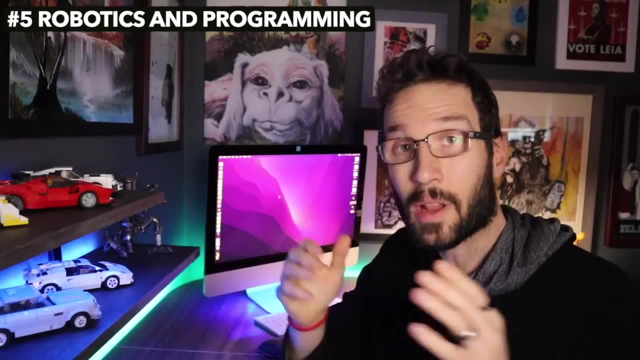 for modeling and analysis of engineering systems. Other topics include loops, functions, image processing sensors, microcontrollers and mechatronic systems. So last up in this category we have mechatronics. In mechatronics, you're gonna learn everything: robotics, right. 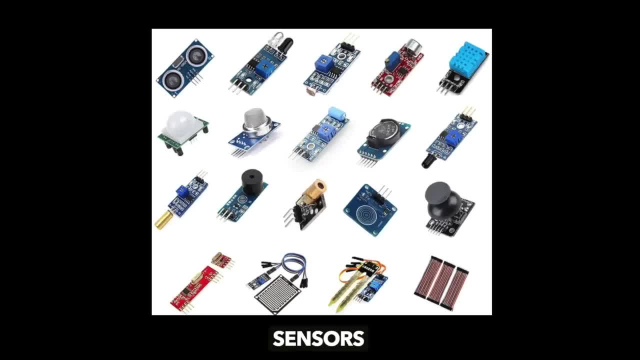 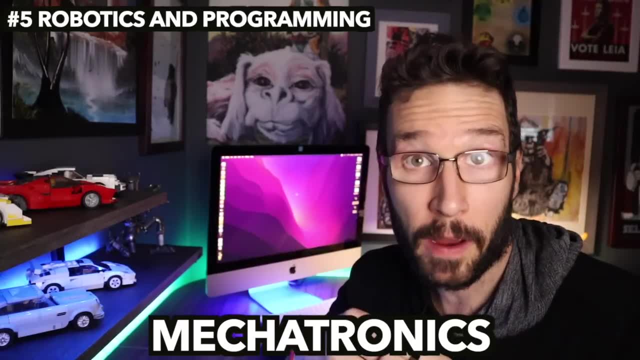 Linkages, control systems, microcontrollers, sensors, actuators, programming servos and motors. Mechatronics was really one of my personal favorite courses because it was really where I felt like all my knowledge was coming together into something really useful. 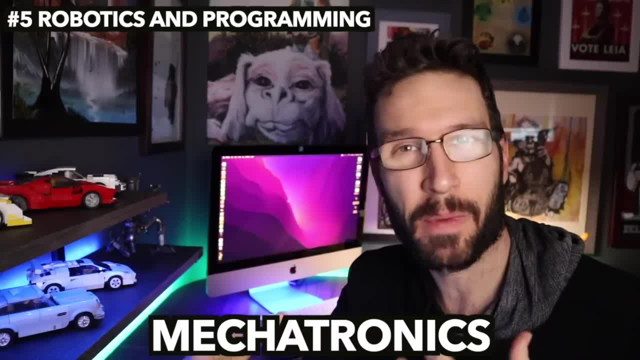 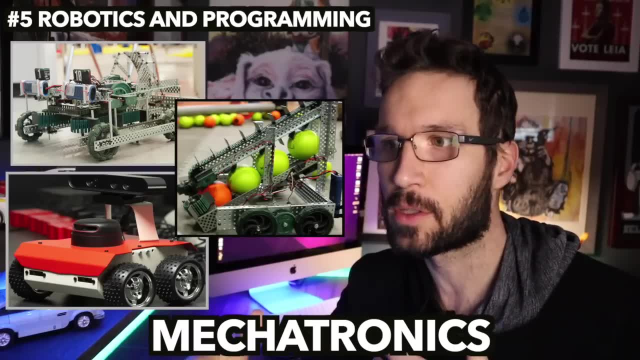 And then to add to that, mechatronics is usually project-based, which makes it really fun. So you'll design and build a robot throughout the course, And the robot is supposed to perform some kind of special task or compete with the other robots in your class at the end of the year. 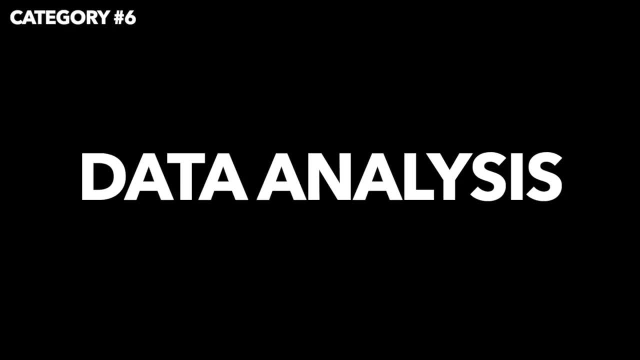 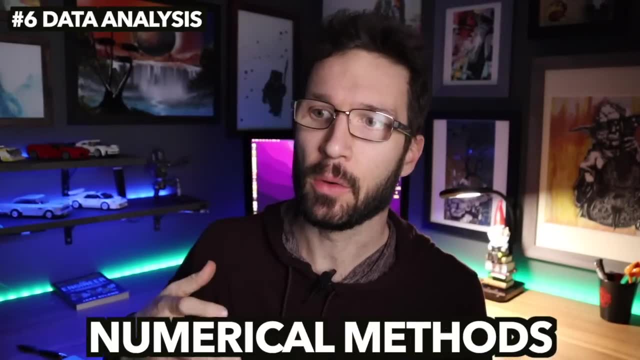 Super fun. Category number six: data analysis. So first up in this category we have numerical methods. So in numerical methods you're gonna learn all about. you know how to create and utilize computer programs that you make to solve some pretty complex engineering problems. 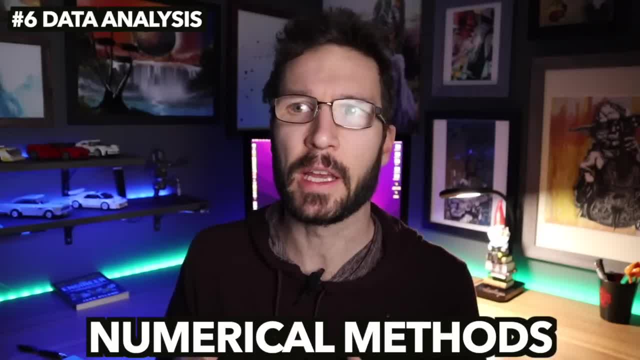 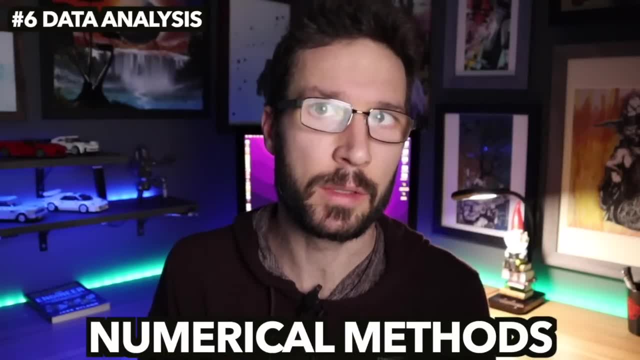 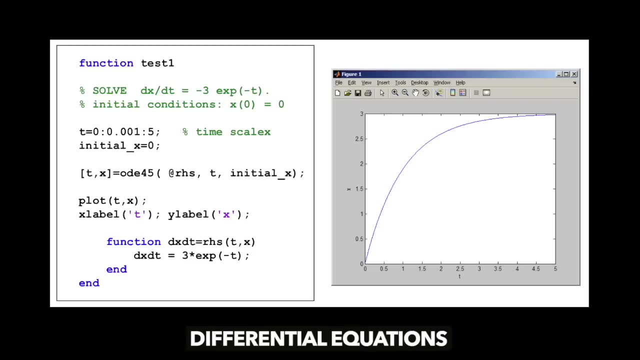 This class is pretty tough, but it's pretty fulfilling in that it shows you how to build your own tools through computer programming and computer programming to solve some pretty hard problems. So some of the topics include root finding, interpolation, approximation of functions, integration, differential equations. 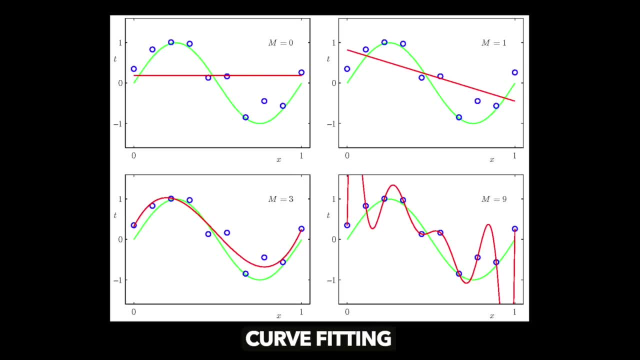 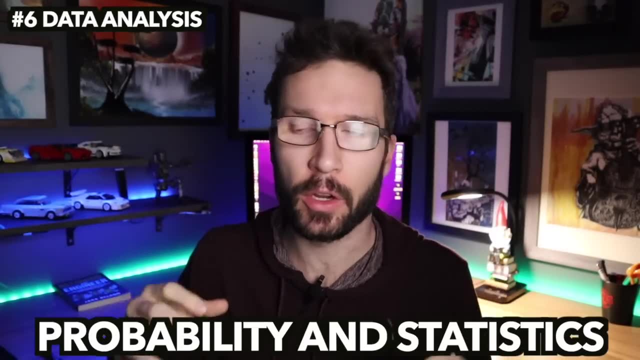 direct and iterative problem solving and curve fitting. So next up in this category we have probability and statistics. So in this class you're gonna really learn how to deal with large amounts of data. You're gonna learn how to utilize statistical methods. 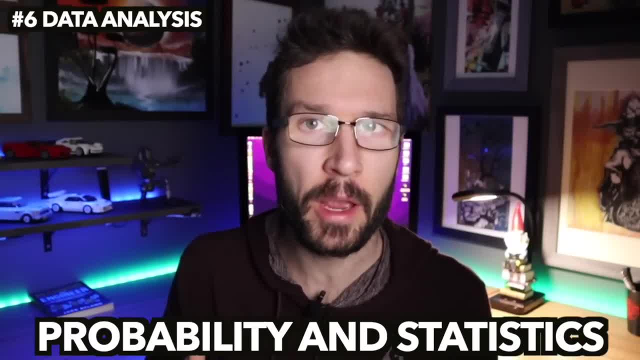 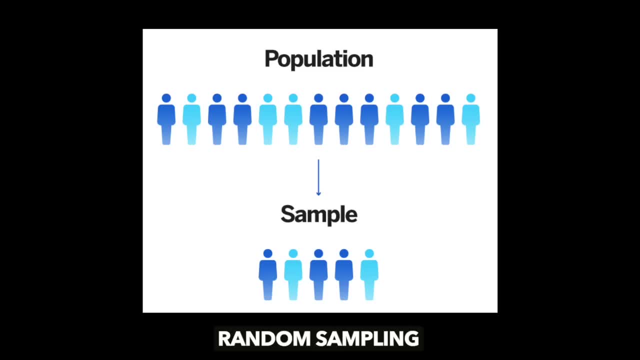 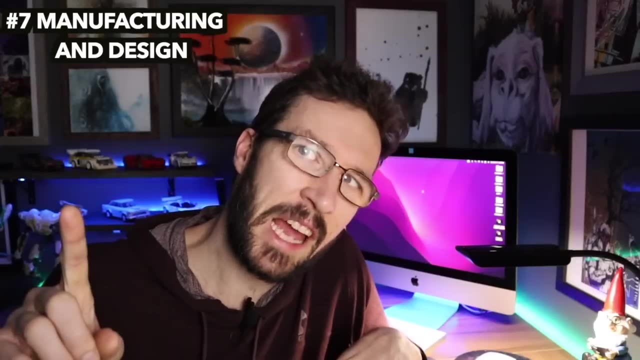 and programming to find trends and useful information within large amounts of data. Other topics include probability theory, distributions and random sampling. Okay so, lastly, we have category number seven: manufacturing and design of mechanical systems. So first up in this category, we have manufacturing. 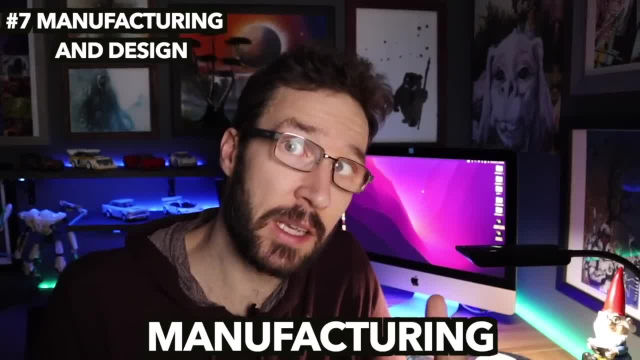 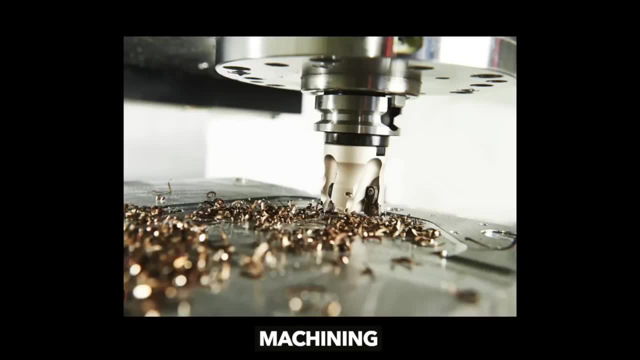 So in manufacturing, you're gonna learn all about the different manufacturing processes and how they're utilized on all the different materials. In this course you're also gonna learn about material removal or machining, material forming, like bulk deformation, and sheet metal forming, casting, polymer manufacturing. 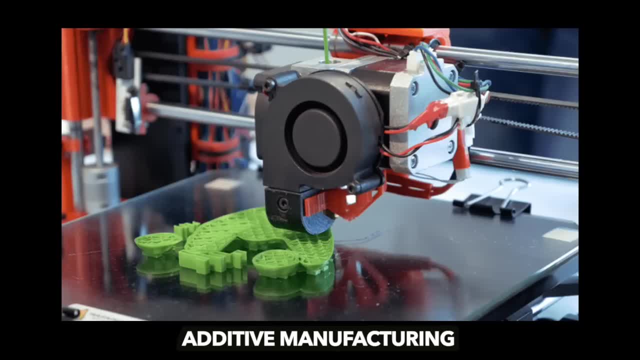 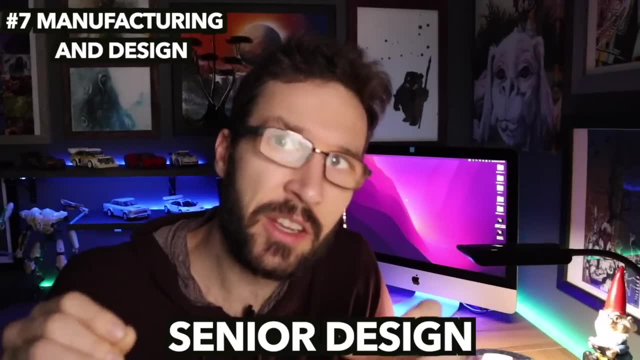 composites manufacturing, welding, additive manufacturing, micro and nano manufacturing and quality control. So, lastly, we have senior design. So senior design is kind of where it all pays off right, Where you can kind of spread your newly formed engineering wings, so to speak.